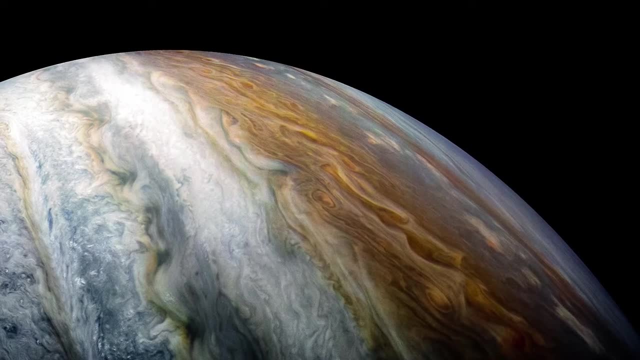 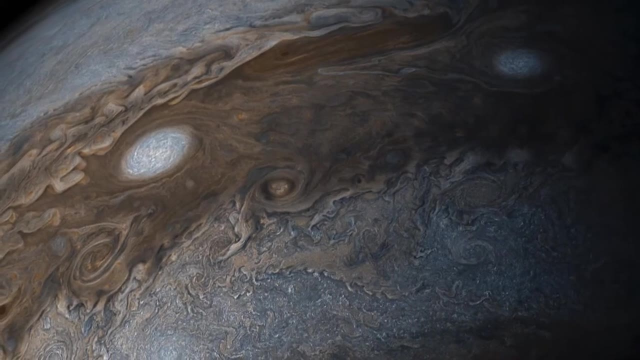 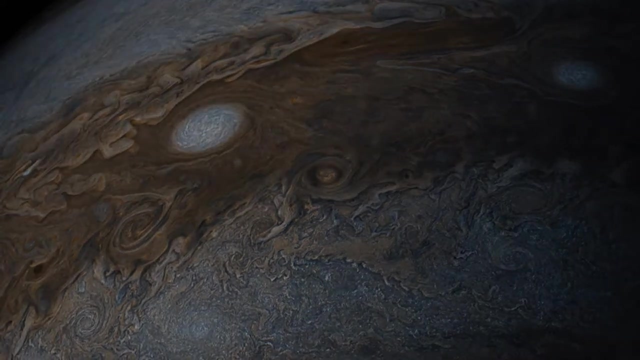 if it's not in a solid form, the material that planet composed of- and we know that many outer planet has semi-liquid or even plasmic type of surfaces- They still might retain the gases on top of it which we call atmosphere or not, for example, like Mercury. Let's see which parameters of 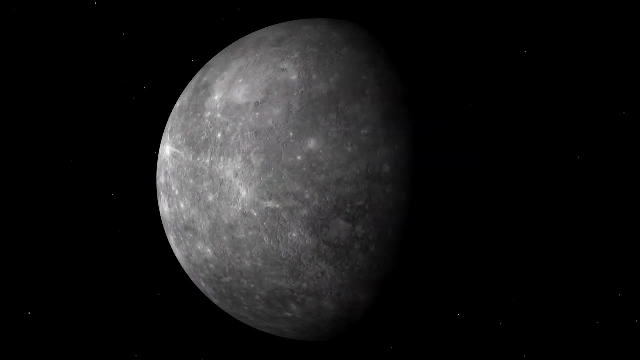 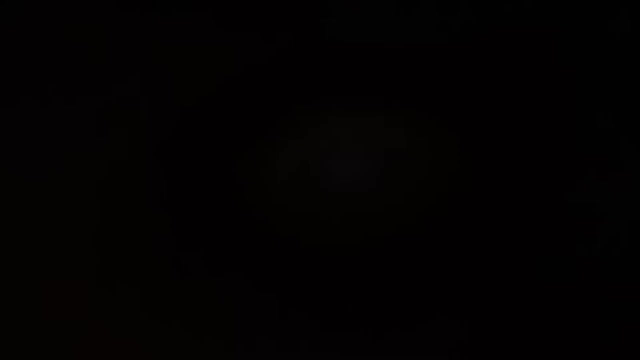 the planet will determine if this layer of the gazes will stay in its surface or not. First of all, we need to talk about the types of atmosphere we can find on a planet. The gazes, which differentiate between each other, are differentiated during the formation of the planet. When the planet 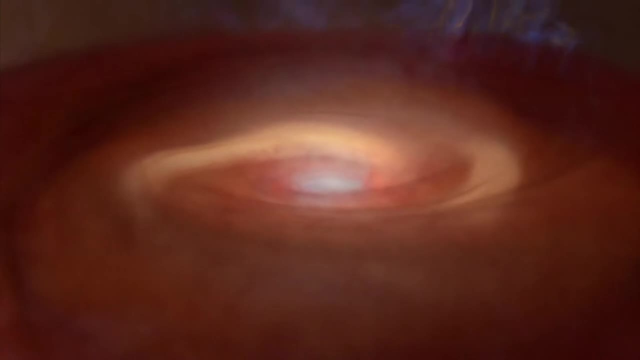 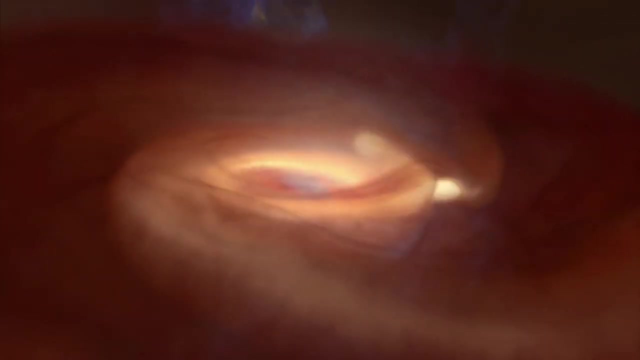 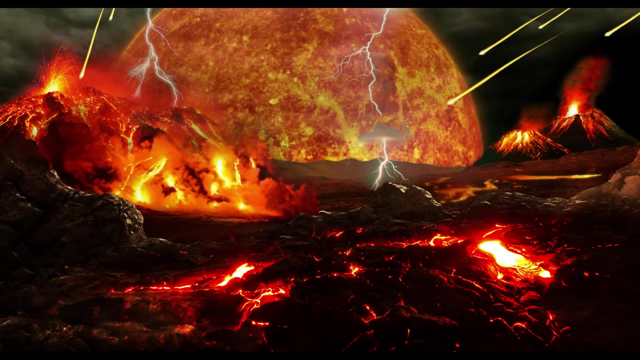 was formed, it was condensing more heavier materials, elements were going towards its bottom or surface and the gazes stay all around it. At the same time, we can have the atmosphere which formed during the lifespan of the planet, and we call it odd gazing. It's the gaze which come from the interior of the planet through 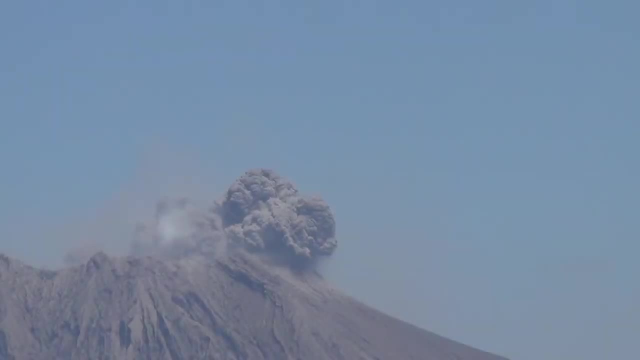 its life. For example, our planet have a lot of water vapor in the atmosphere, hydrogen oxygen and other elements, carbon dioxide, which come out during the degazing through the volcanic activity. In case of the Earth, we have the atmospheric composition change through the life forms developed on our planet and it 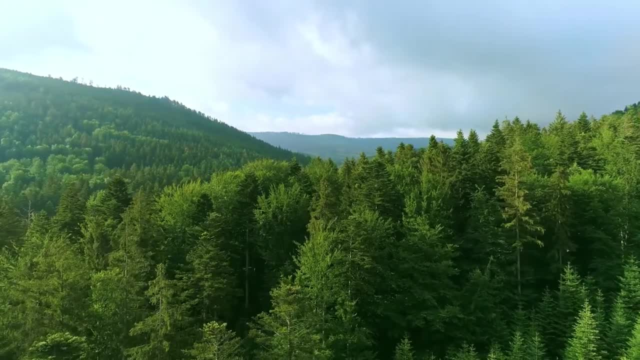 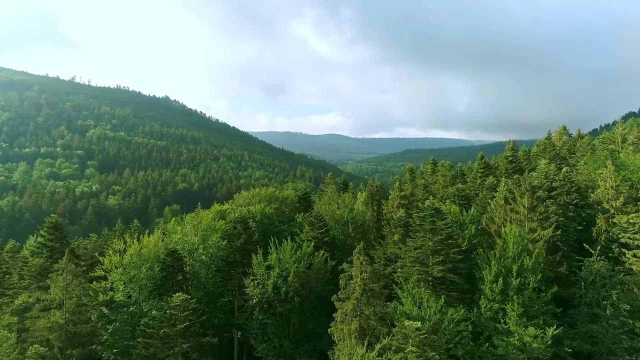 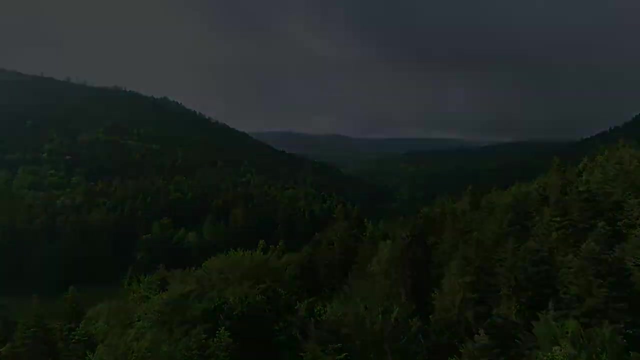 won't be the primer atmosphere, it will be secondary or further atmosphere of that particular planet. So what determined for the gas to stay on the surface of the planet or not? As you remember your basic physics classes, each of the molecular moves in form of the gaze, the molecular vibrate and move with particular speed. We call 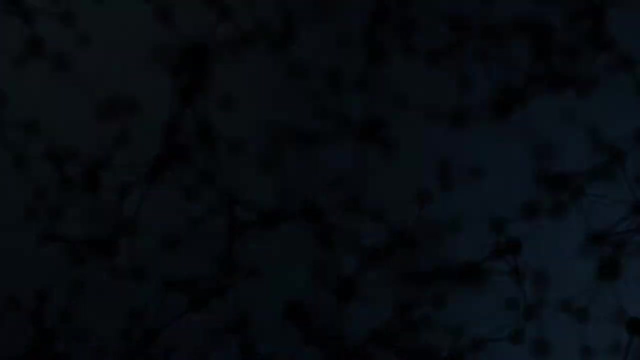 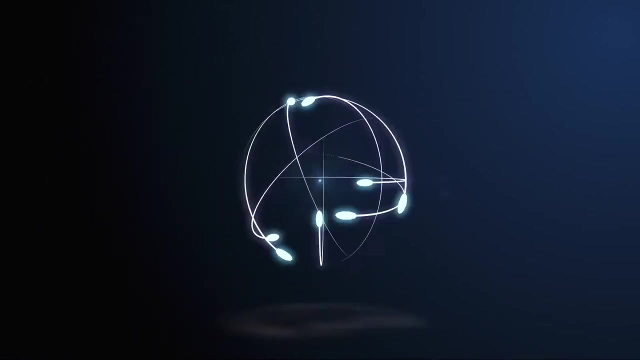 it. molecular speed: The speed of the molecular: how fast it will vibrate. spin will depend on its mass: how many protons neutrons in an atom, how big the molecule and how complex. In the previous videos about radiometric dating and 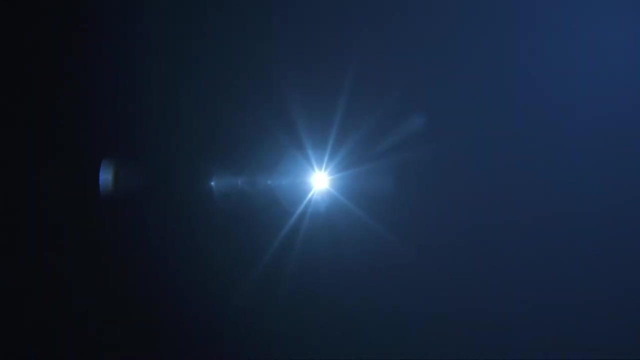 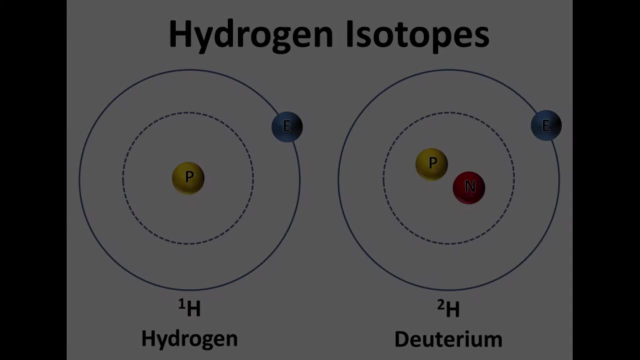 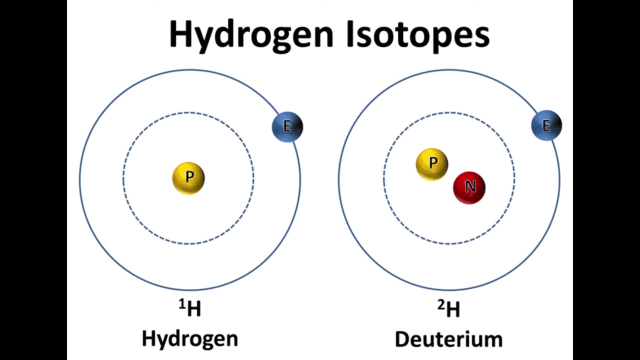 climate proxies. we talked about these properties of the molecules. for example, hydrogen have one proton or one proton, one neutron, and its mass is very low. so the molecular have quite high speed and with increase of the temperature it will increase its speed faster. therefore, for example, like on our planet, we don't have 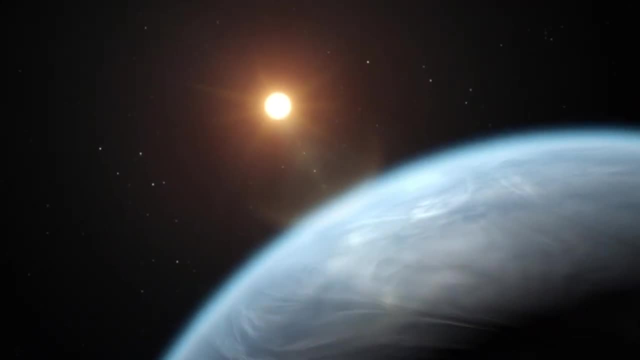 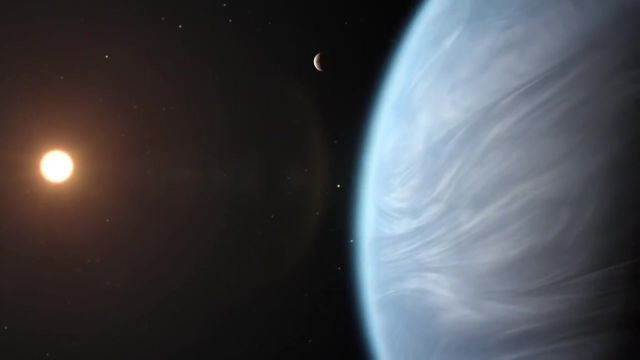 much free hydrogen in our atmosphere because it's vibrate very fast and if it's reached the high levels of the atmosphere, this molecules, and if the direction of the movement will be pointing away from our planet, the molecular of the hydrogen will just escape our atmosphere and go into the space. but the mass molecules all stay around our planet by the forces of gravity. so of course, the bigger the radius of the planet, the denser the planet, the bigger gravity will be on this planet. so the gravity will be one of the parameter will influence the atmosphere composition. 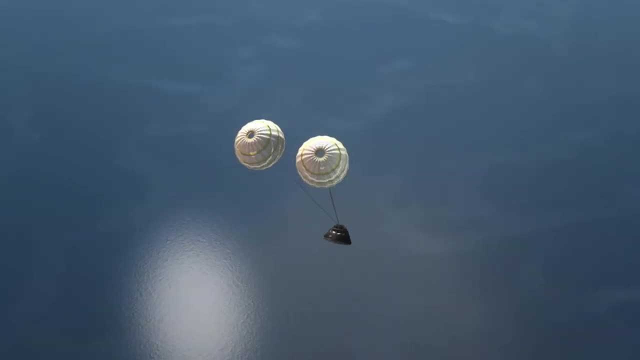 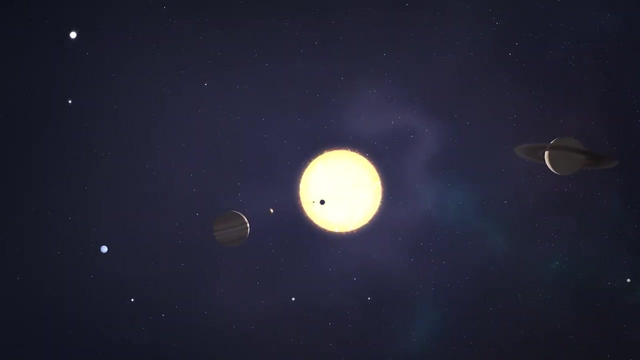 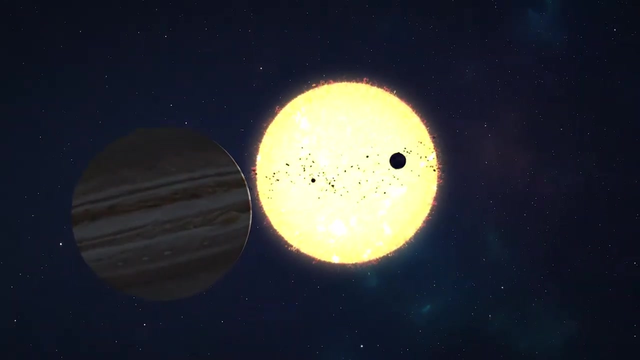 thickness and if you have atmosphere at all. and, as I said, temperature will affect the speed of this molecules as well. so if your planet is closer to the Sun, obviously we have higher temperatures on the surface. it will mean that it's easier for lighter molecules to escape the atmosphere of that planet. 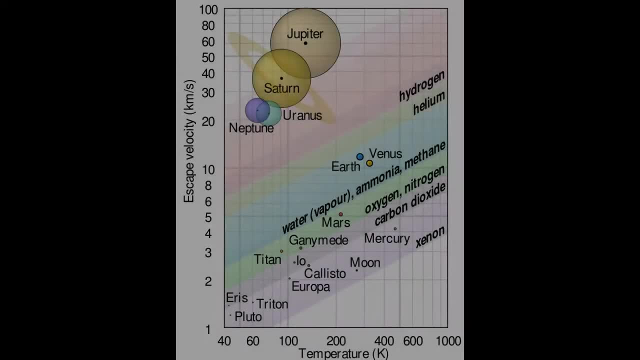 in summary, you can easily calculate, knowing your expected molecular speed. for example, for hydrogen it will be one number, for heavy molecules like oxygen or two, it will be higher number. mass weight will be 32 rather than one or two as for hydrogen. therefore, you can. imagine the oxygen have more possibilities to sunk down towards the bottom and stay in the atmosphere than lighter hydrogen. with high temperatures will escape it easier. escape velocity as well, depending on the gravity and the radius of the planet. therefore, is my molecular speed will be higher than escape velocity for this particular 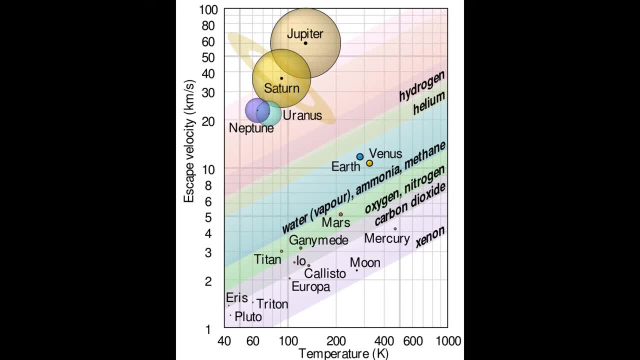 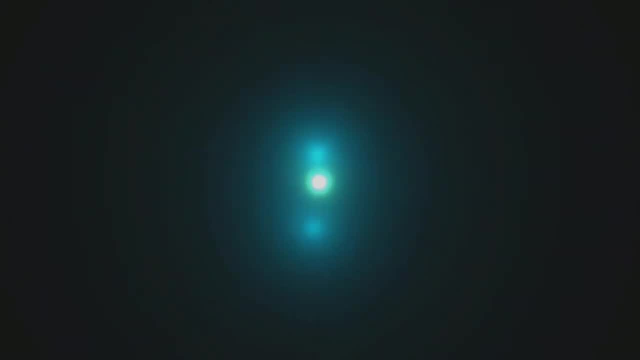 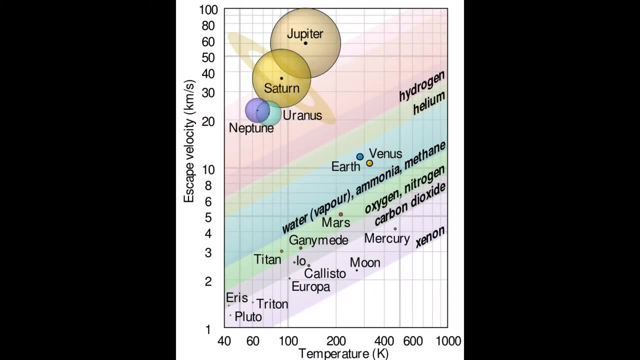 planet which depends on its radius, therefore gravity and mass of that planet. so I will lose these particular atoms. we can differentiate all the molecular gazes in our atmospheres around our solar system, for light gazes, in heavy gazes and depends how far the planet from the Sun, temperature wise, is this. 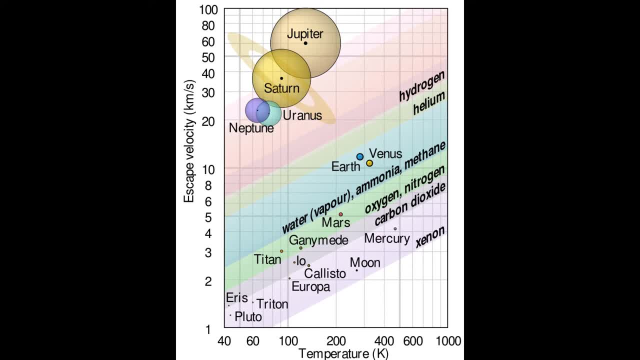 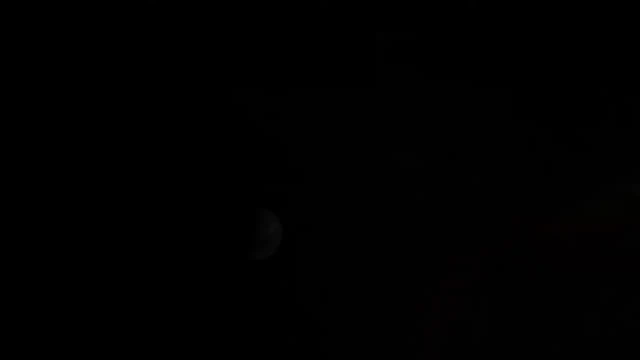 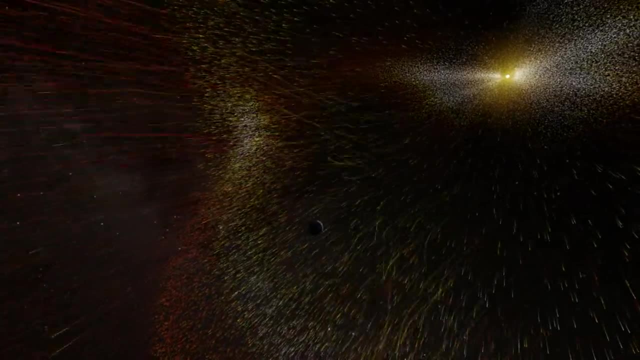 planet is heavy, big gravity. it will retain the atmosphere, heavy and light gazes. we will just retain heavy gazes or non gazes at all. there's other parameters which will affect if you have atmosphere or not, for example, things like solar wind. it's the constant flow of the particles coming. 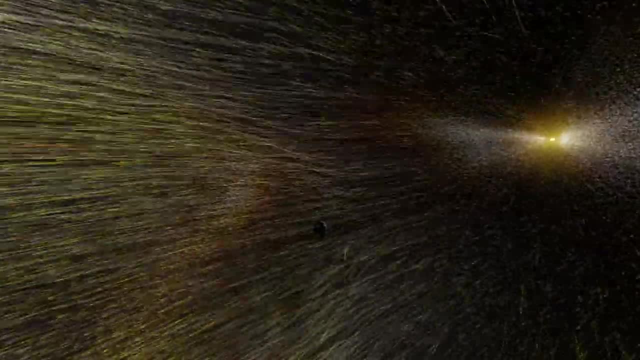 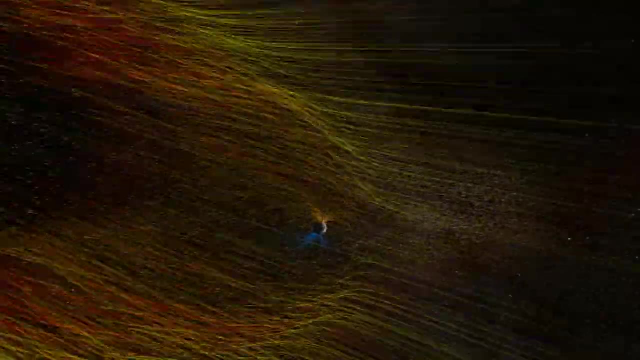 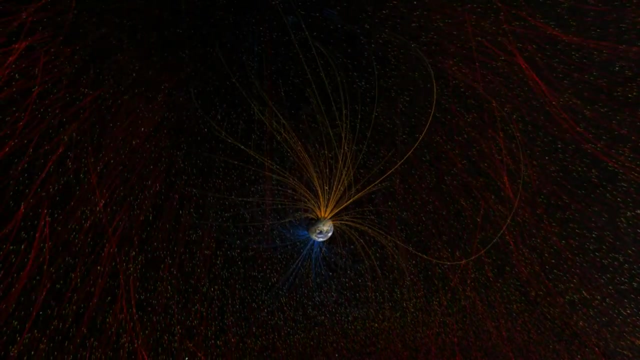 from the Sun- we call it solar wind- and if they're strong enough they can swept away the light gazes on high surface of the planet atmosphere away into the space. we know on our planet Earth we have strong magnetic fields which produced by our core, metal core. if I didn't have the metal core, when you have the strong, 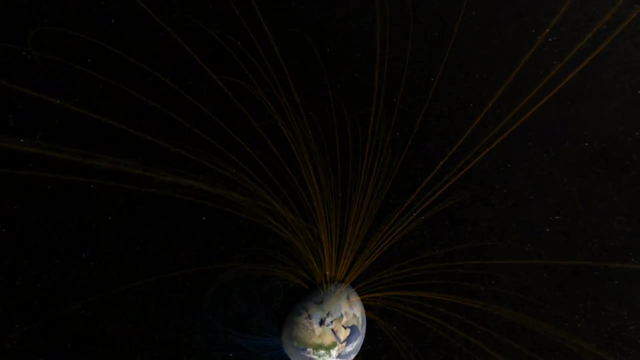 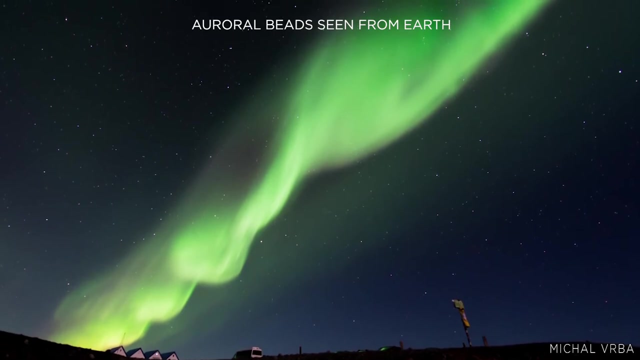 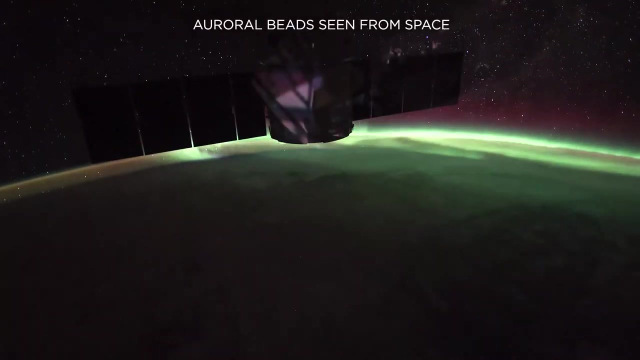 magnetic field around my planet and let's protect us from this wind of solar energy will semi protect our atmosphere for being swept away. we're all seeing the Aurora in the northern areas of our planet. this is the particles of the solar wind share against our high levels of atmosphere. 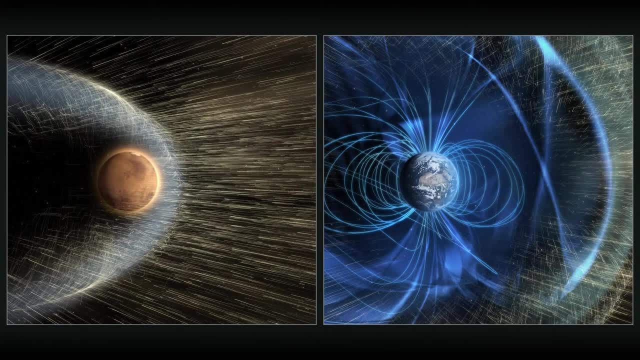 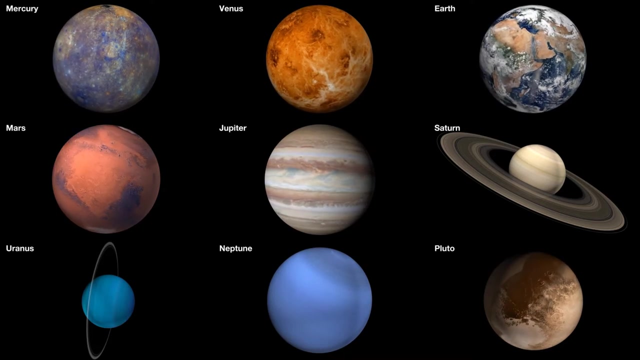 For example, on Mars, sparse molecules of the gases which retain on this weak surface due to the very low, almost non-existing, magnetic field, swept away by the solar wind very easily. Therefore, we can rank all our planets depends on these properties and see which atmosphere they. 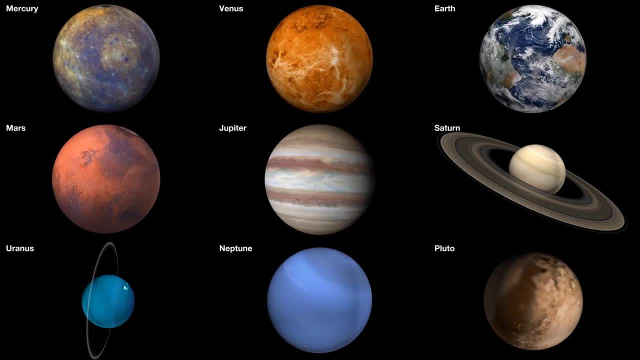 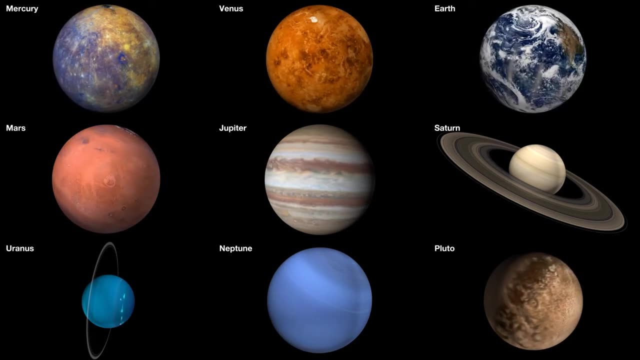 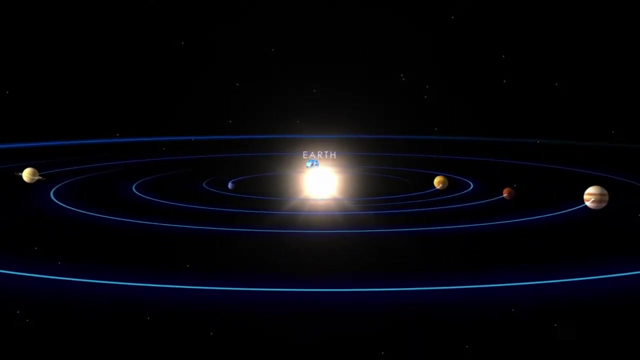 will have at the wheel, dominated by light or heavy gases, or they might not have atmosphere at all. Let's have a look on the order of our planets from the Sun outside to the aegis of our solar system. We start with Mercury. closer to the Sun, Venus, Earth, Mars- We're called inner planets, or 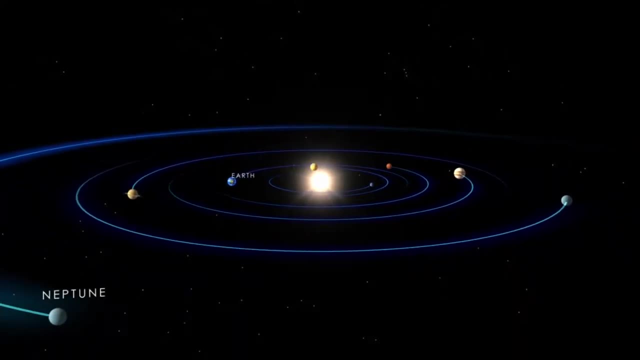 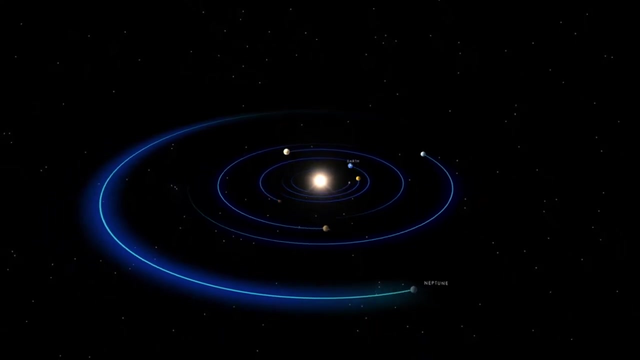 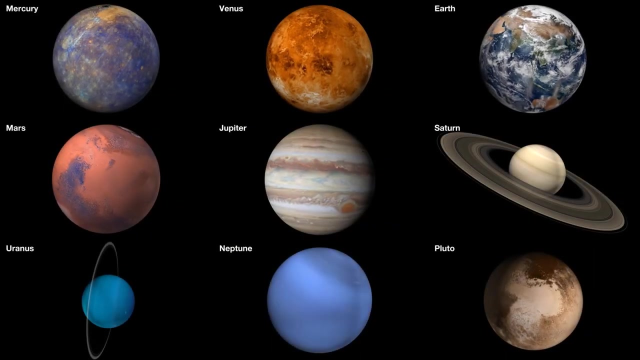 earthy type terrestrial planets And we have huge gases. Jupiter, Saturn, Uranium, Neptune and it used to be Pluto, but it's not categorized the planet anymore. Only the Mercury have no atmosphere at all and we have the Mars with quite sparse atmosphere. Otherwise the rest of the planet have atmospheres, but they differ. 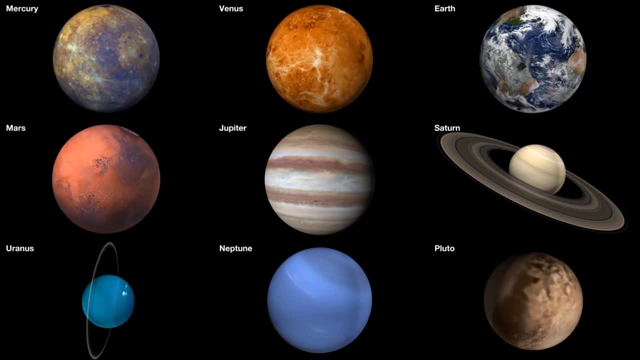 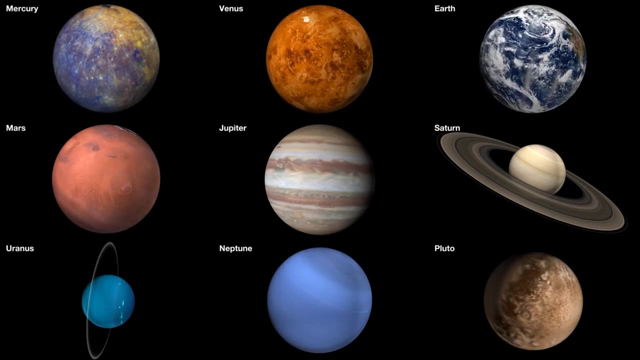 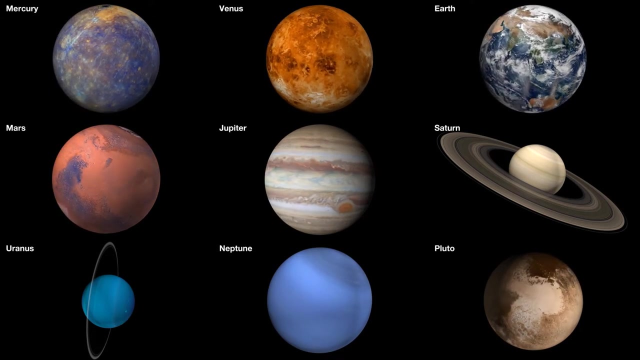 Let's look by parameters, For example, light and heavy gazes, which, as we talked, depends on the gravity of the planet, its radius, its size and the speed of these molecules. Lighter molecules, as I say, have high speed and they're easier to escape, and the heavier gazes, they stay longer. 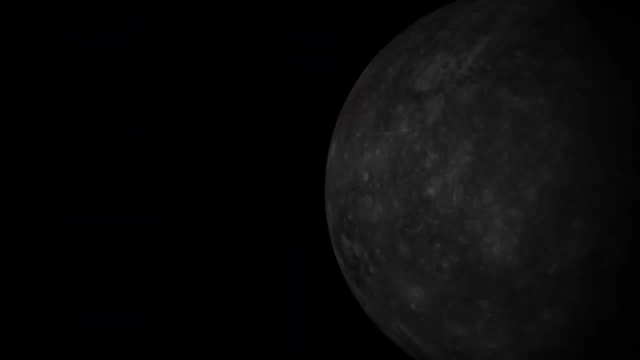 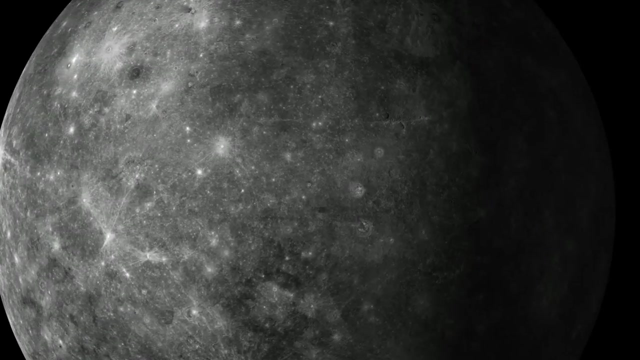 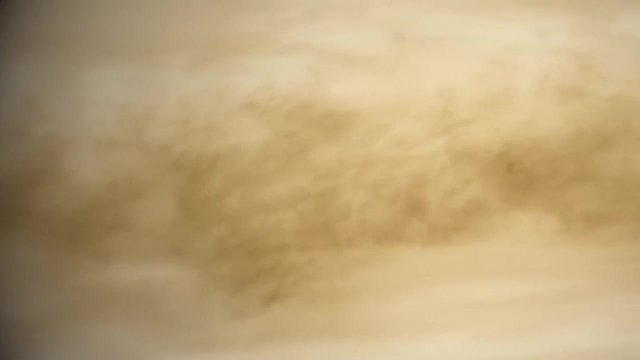 because they're heavier and they move a little bit lazier, slower. So Mercury is so close to the Sun, it has very high temperature on its surface. as light and as heavy gazes they both escape it, So we don't have atmosphere left. Venus has very thick atmosphere, but again the light gazes 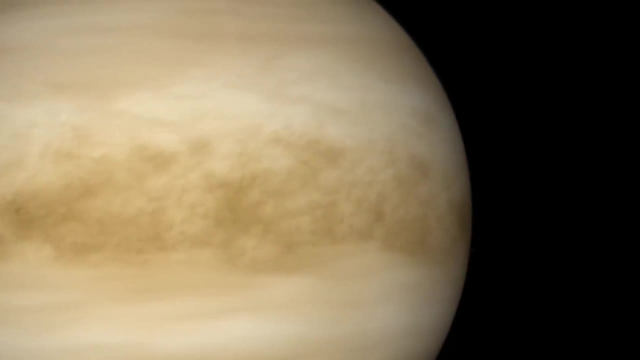 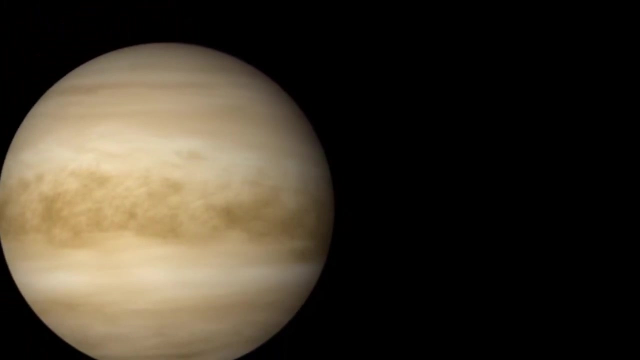 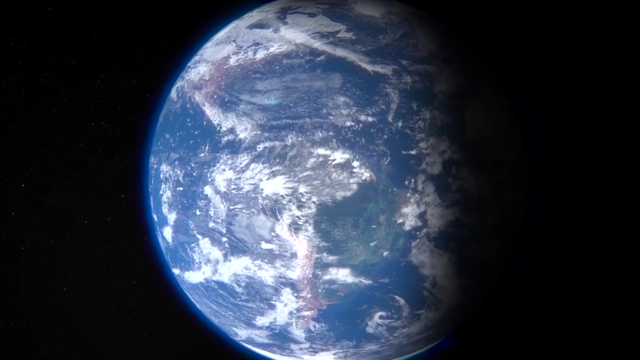 escape it. if you calculate its escaping velocity And the speed of the light molecules, We have only heavy gazes left, And the atmosphere on Venus is very rich with carbon dioxide and it's hot. Next planet will be Earth. We know our atmosphere: it's dominated by heavy gazes again, but the temperature is. 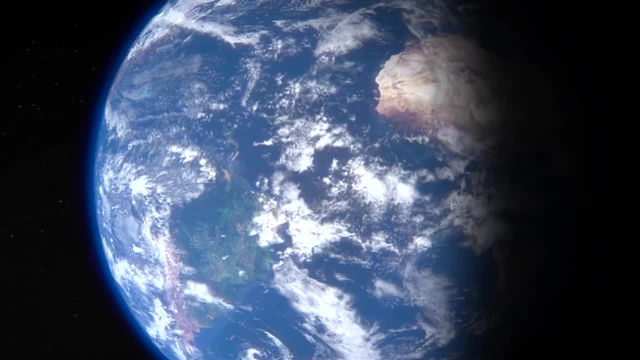 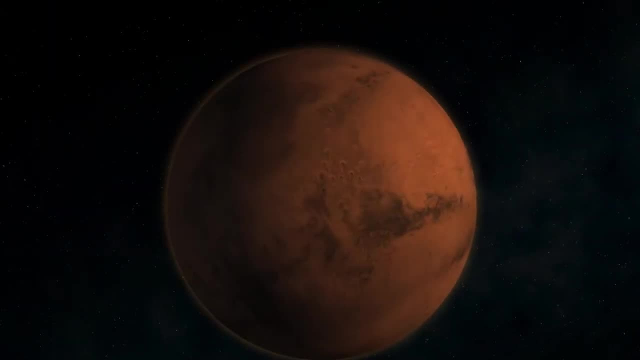 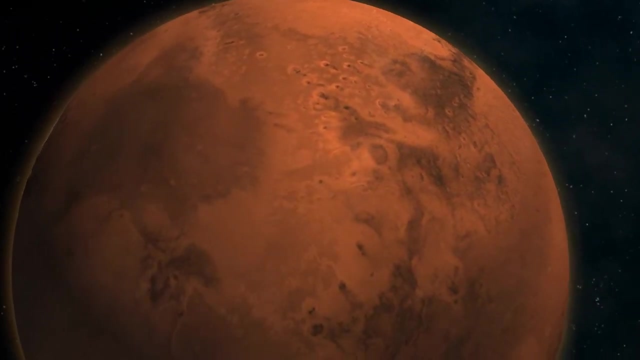 not as hot, so it's okay for us to live on. It's dominated by nitrogen and oxygen. Mars has very sparse atmosphere dominated by heavy gazes, again mostly carbon dioxide. The temperature is a little bit cooler than on Earth and you can figure out the radius of the 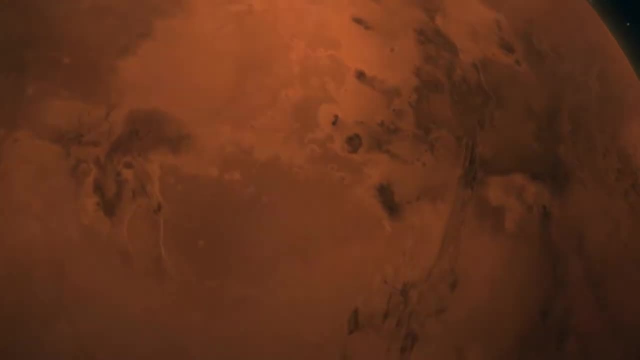 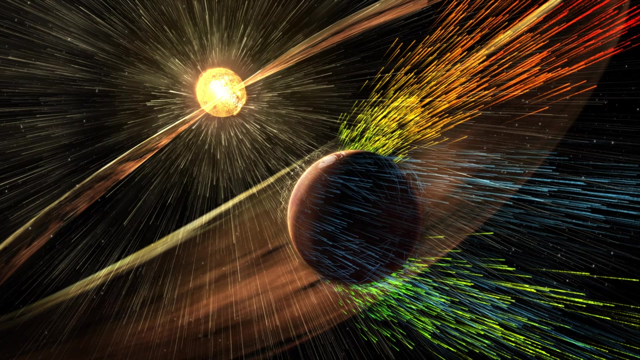 Mars much smaller than the Earth and we almost don't have any magnetic field on it. So therefore the Mars easier lost its gazes on its surface. It's very, very sparse atmosphere for us would be almost impossible to breathe, and it's very much sensitive to the solar wind. All these 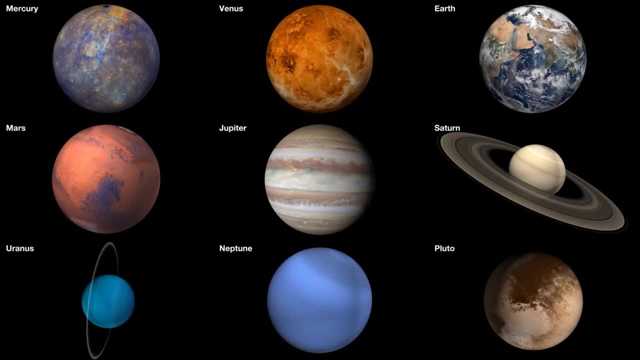 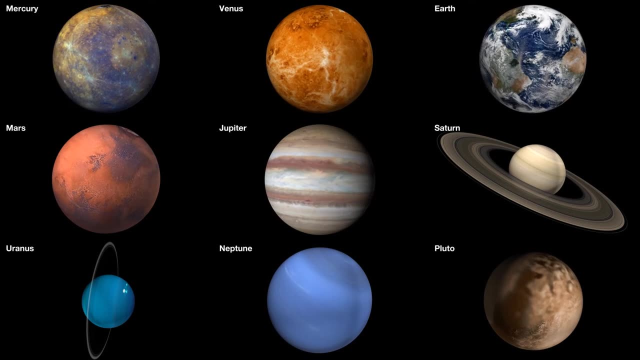 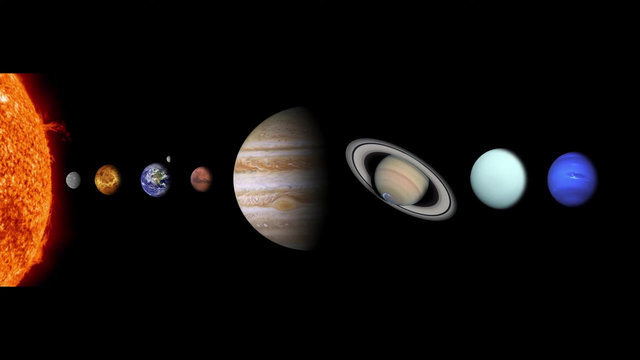 four planets have slow rotation, they all have solid surfaces and they have temperatures from hot to temperate. Next outer planets: It's the huge gas planet we recall because of that, because mostly they're composed of dominated gazes and heavy and light gazes. 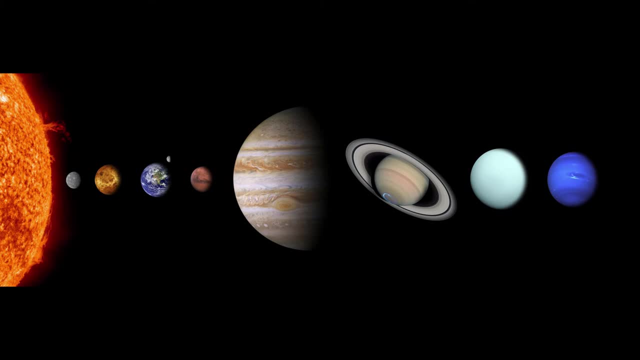 This planet's quite far from the Sun. the temperature on its surface is lower, so they can retain those low gazes. Plus they have bigger radiuses. They don't have any solid surfaces. so if you go on the surface, for example, of the Jupiter, you kind of will sink into something between gaze. 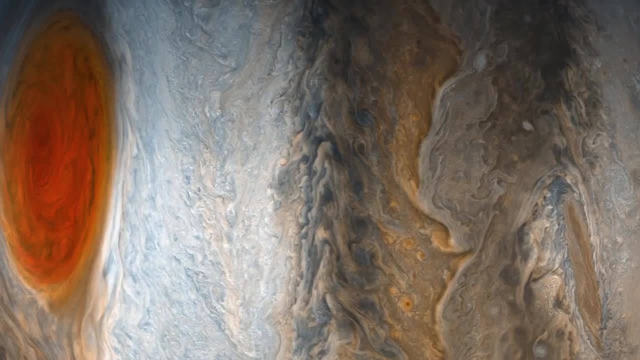 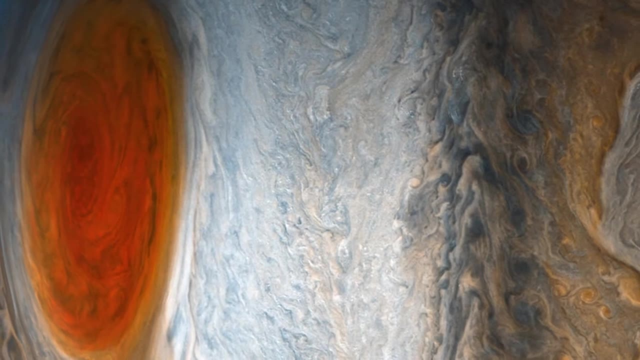 or plasmic state. All these planets are rotating quite fast- it'll be surprising to know- And they have as heavy gazes in the composition as light like hydrogen helium. They have lower density than our solid terrestrial planets and much colder. 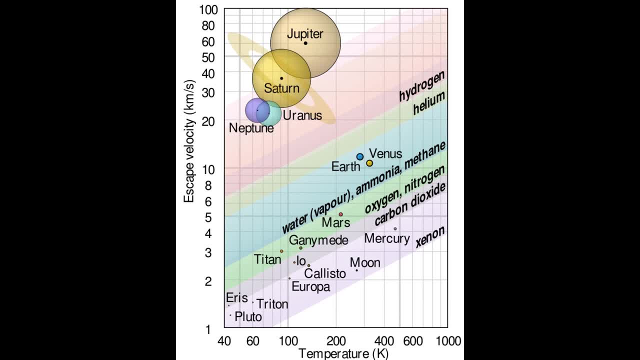 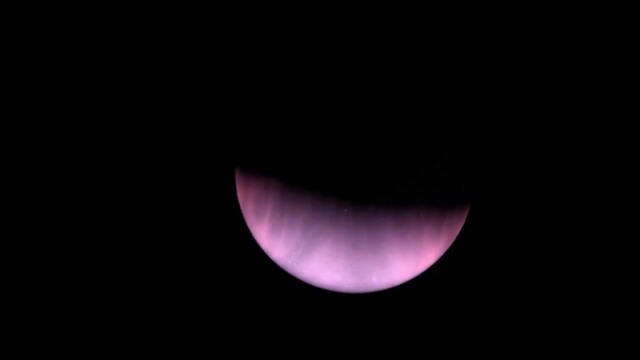 temperatures. And for sum up, we can see Mercury doesn't have any atmosphere. Venus have rich carbon dioxide atmosphere, with clouds dominated. that's why this planet is very bright, One of the brightest planets in our solar system. You can see it later in the morning. 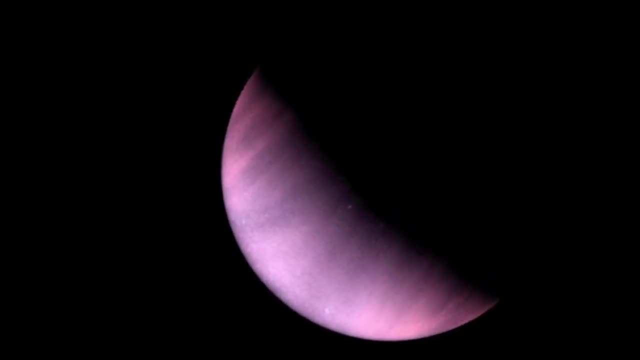 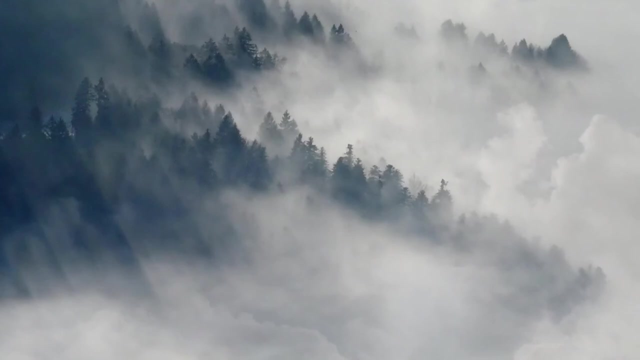 and earlier than anything in the evening. We know that atmosphere very hot there and green house effect is very strong. Earth nitrogen, oxygen composition of the atmosphere: it's half water, partially. not like Venus. we don't have thick layer of the cloud all over the planet. 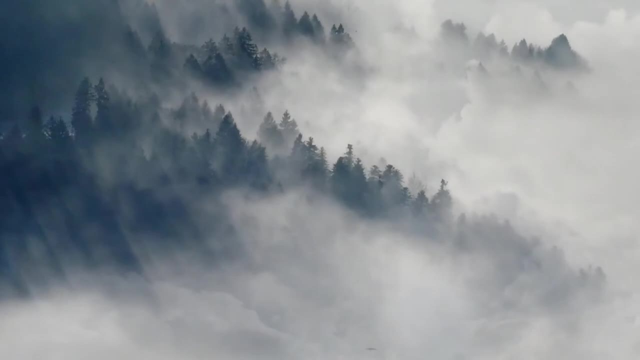 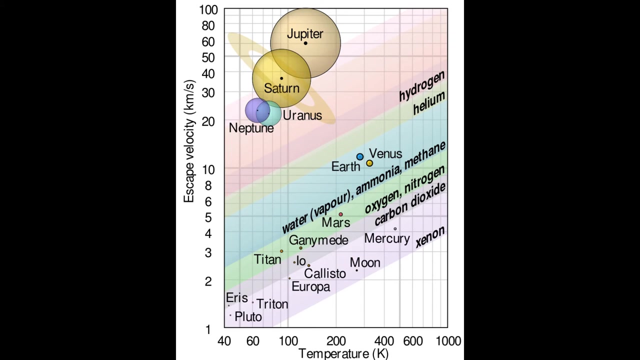 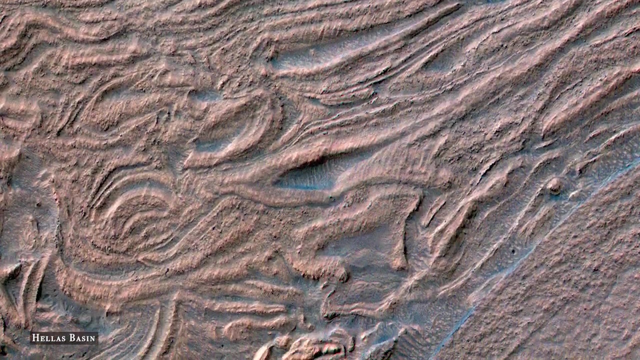 surface But we have things like ice caps and the life forms on our planet, Mars. Mars has very sparse, low density carbon dioxide atmosphere. It have some ice caps but they not made of the water molecules but the carbon dioxide molecules- dry ice.